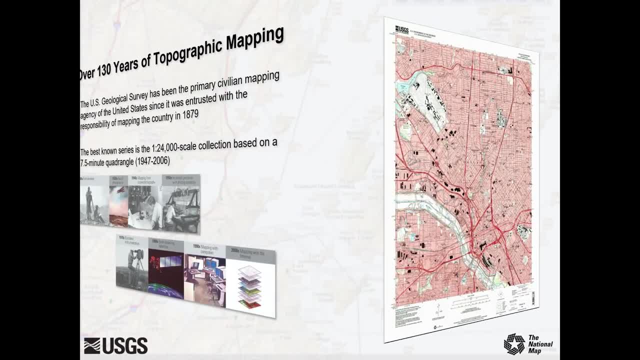 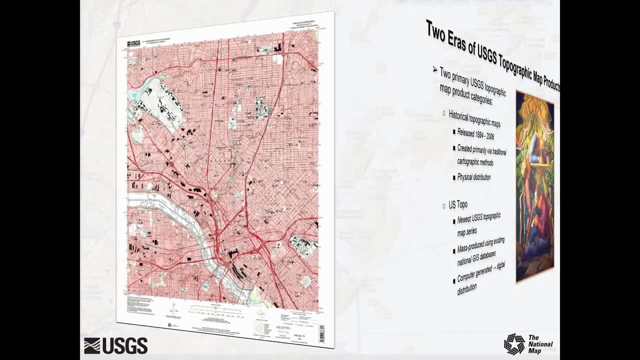 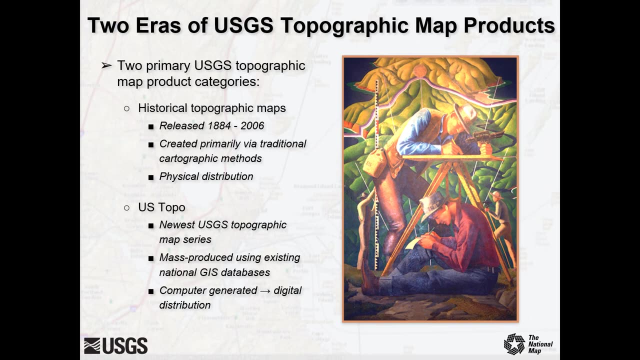 updated through 2006.. The 1995 Dallas Texas map seen here is a modern example of the 1 to 24,000 scale map series USGS. topographic maps can be categorized into two primary products. The first is the set of maps released between 1884 and. 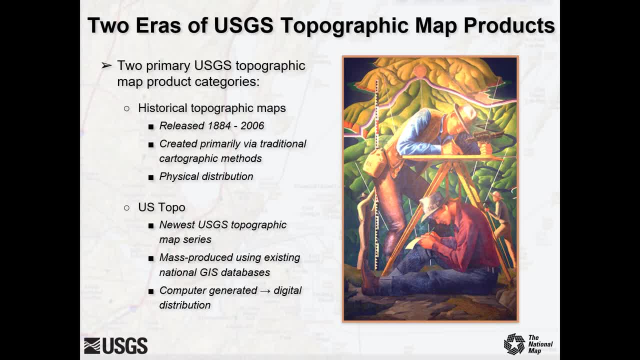 2006.. These older, more traditionally created topographic maps are referred to as historical topographic maps. The release of US Topo, the newest USGS topographic map series, marked the end of that era and the beginning of another for the USGS topographic map products. US Topo maps are digitally mass-produced. 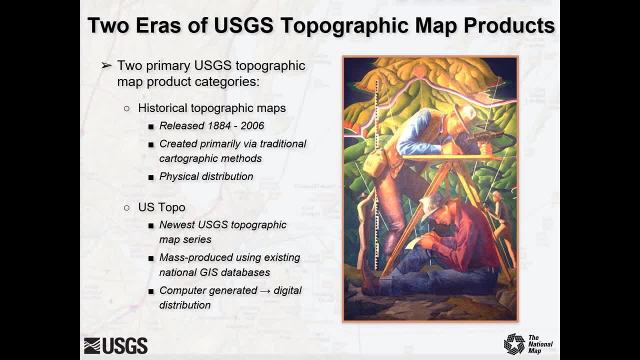 using geographic information system, or GIS databases. These databases stem from the national, state and local partnerships established as part of the national map which you learned about in lesson 2.. How to access both products will be covered later on in this lesson. First, we 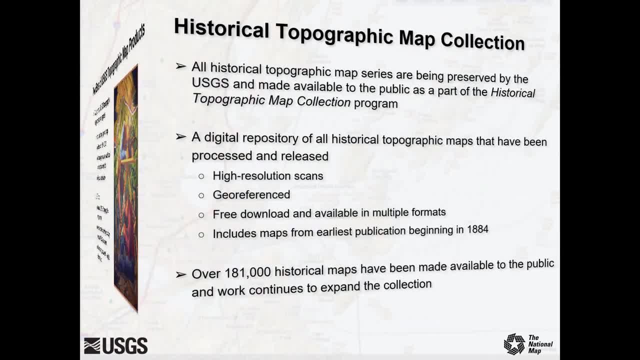 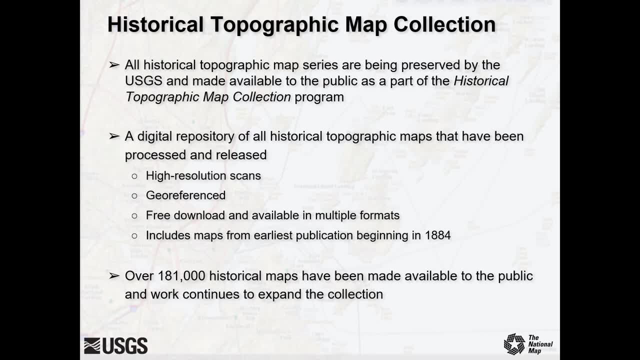 will focus on the historical topographic maps. The USGS has overseen an effort to preserve the maps and make them available for online download. This is known as the historical topographic map collection, or HTMC. HTMC is the group of all USGS topographic maps created before US Topo. The goal has been 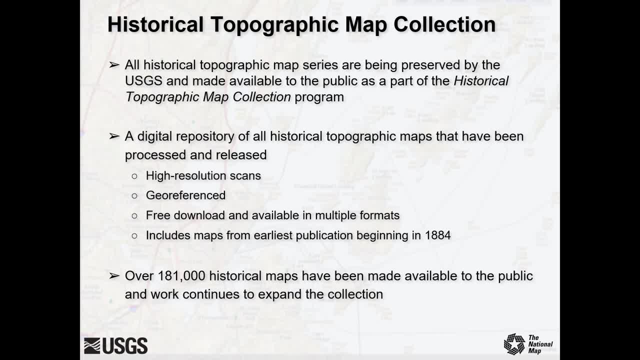 to include every historical USGS topographic map since the first series, which began publishing in 1884, and over 181,000 have been scanned so far. The USGS has also been able to include all USGS topographic maps since the first series. 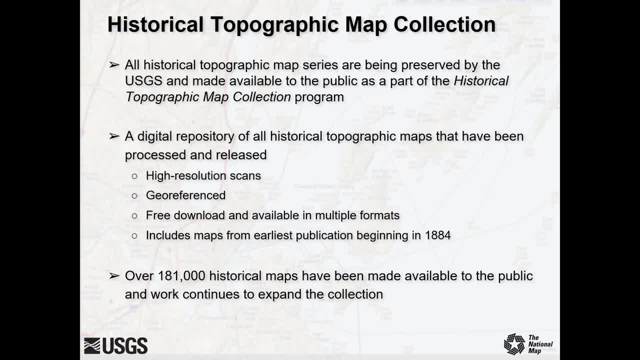 which began publishing in 1884, and over 181,000 have been scanned so far. The goal has been to include every historical USGS topographic map since the first series, which began publishing in 1884, and over 181,000 have been scanned so far. Every scale with a priority on the 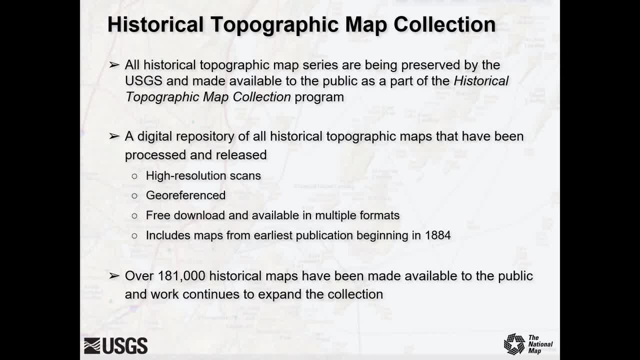 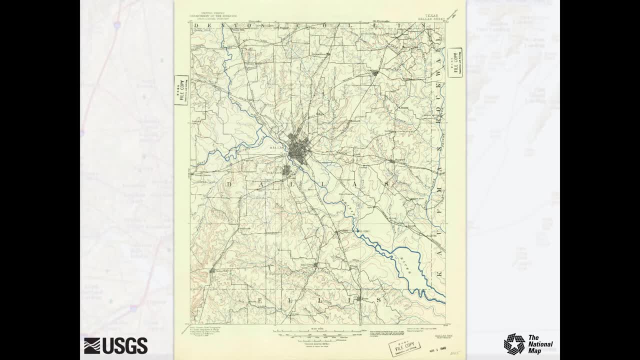 traditional 1-24,000 scale maps and addition is being scanned at a high resolution and made available for download. Seen here is a USGS Topographic Map of Dallas, Texas, published in 1893.. It is an example of one of the earliest USGS topographic maps and is available to the public through HTMC. 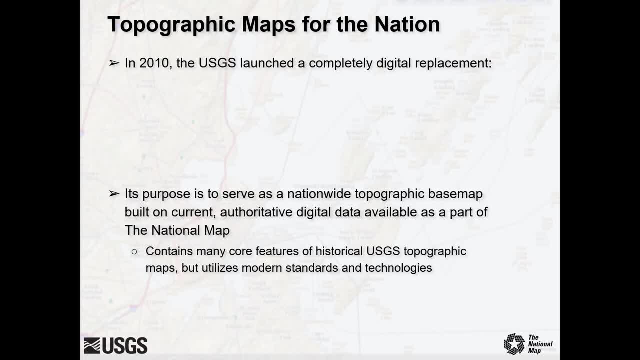 In 2010,, the USGS launched a completely digital replacement topographic After extensive preparation and testing. the new map, which will offer national coverage of all states and territories, is called US Topo. The purpose of the US Topo Map series is to serve as a nationwide topographic basemap. 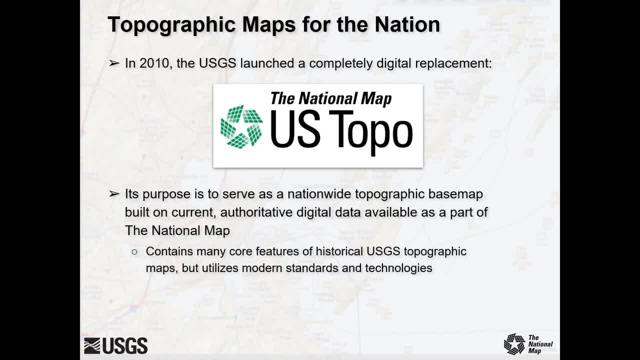 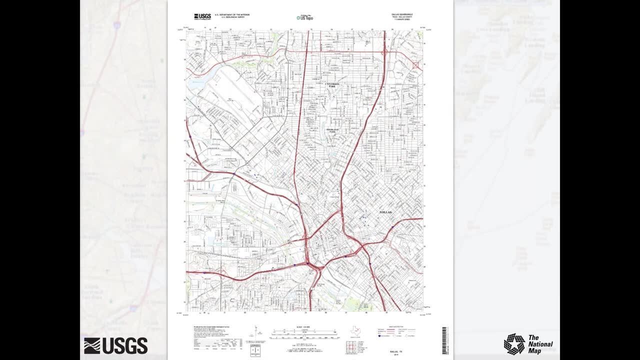 built on current authoritative digital data available as part of the national map. The US Topo maps contain many core features of historical USGS topographic maps, but make use of modern standards of technology. This 2019 map is an example of the latest iteration of US Topo for the Dallas- Texas. 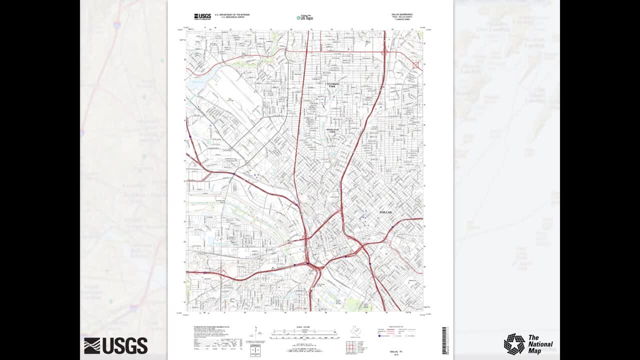 area. One of the easiest ways to distinguish a US Topo map from previous series is the US Topo logo at the top center of the map. As you can see, several types of transportation are included, as well as a green-tinted woodland. 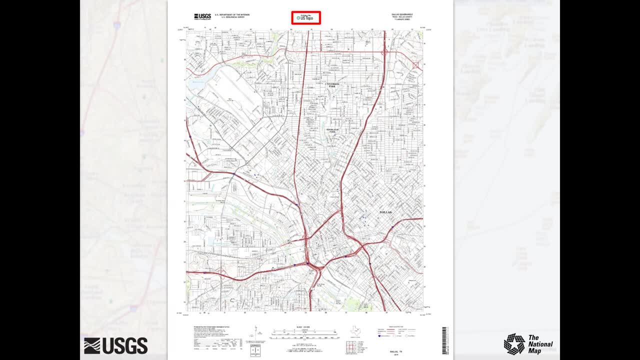 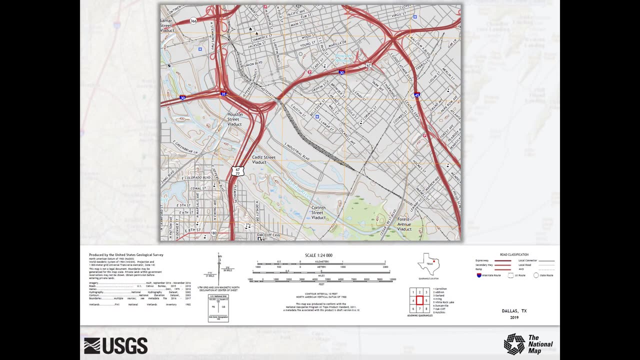 vegetation, land cover- a familiar component on earlier maps- and hydrography or surface water features such as ponds and streams. A closer look reveals the contour lines and geographic names. The gray layer now visible is the shaded relief. DEM or digital elevation model. 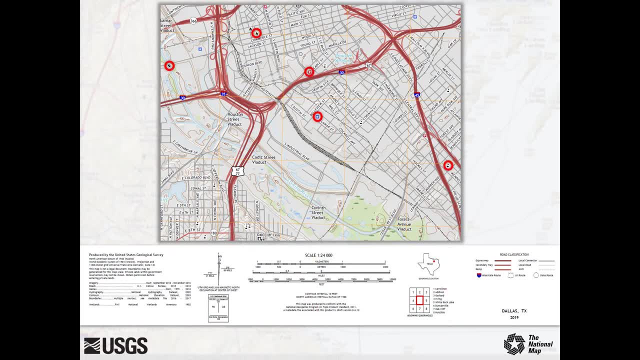 State, county and national boundaries are shown, in addition to limited structure types. The footer of the US Topo map also has a layout similar to previous series, with brief metadata on the bottom left, multiple scale bars in the center and the map name and date on the. 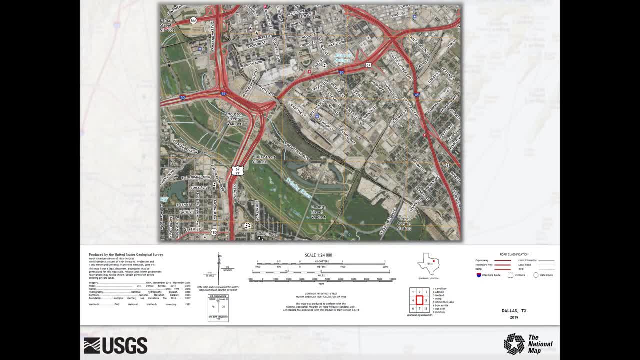 bottom right. New to this series is a recent aerial color ortho image. Although US Topo is not a topographic map, it is a map of the US Topo. US Topo is a new all-digital topographic map product. 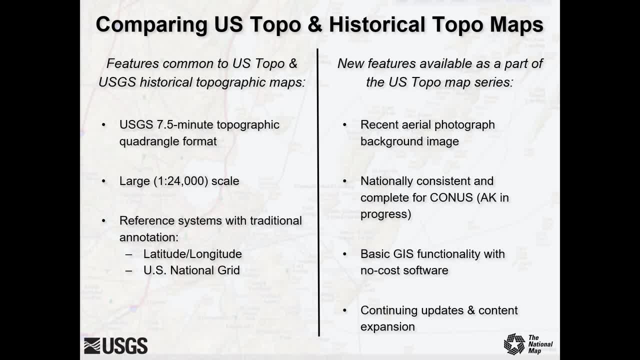 The US Topo maps retain many of the characteristics of the traditional USGS topographic maps, In addition to the similar detailing in the outside margins of the map, it uses the 7.5-minute grid of the earlier map series and has a scale of 1 to 24,000. 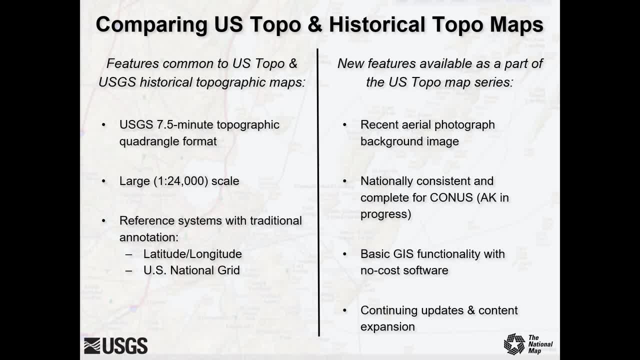 As mentioned before, the digital nature of the product and the layering available in geospatial PDF format allows a recent aerial photo background image to be included. The main advantage of the US Topo map series is that they are nationally consistent and complete for the contiguous United States, Hawaii, Puerto Rico and the US Virgin Islands. 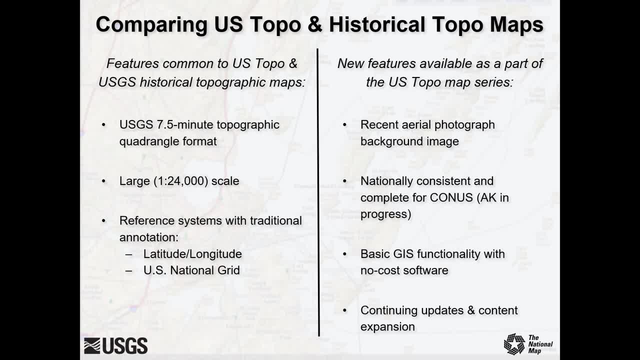 Alaska is very close to completion as well. Furthermore, US Topo maps can be viewed and allow for basic GIS functionality using free software. US Topo maps will also receive updates and content expansions as more data become available. New geographic data layers have been added periodically since the production of the map. 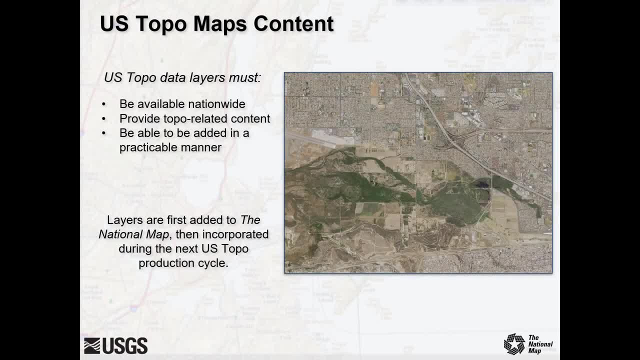 New geographic data layers have been added periodically since the production of the map has been added periodically since the production of the map has been completed, New geographic data layers have been added periodically since the production of the map has been completed. US Topo maps were available until the first US Topo maps in 2009.. 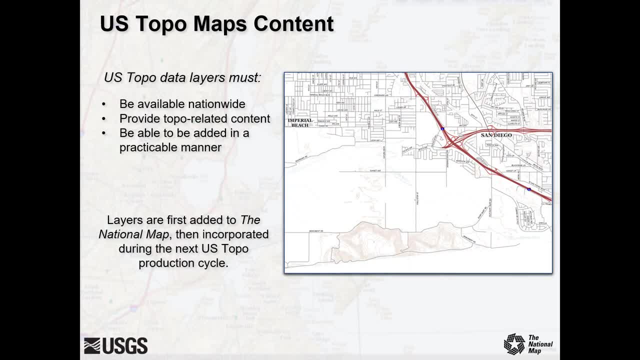 US Topo maps were available until the first US Topo maps in 2009.. In order for data layers to be added to the US Topo, they must be available nationwide, provide Topo-related content and are able to be added in a practicable manner. 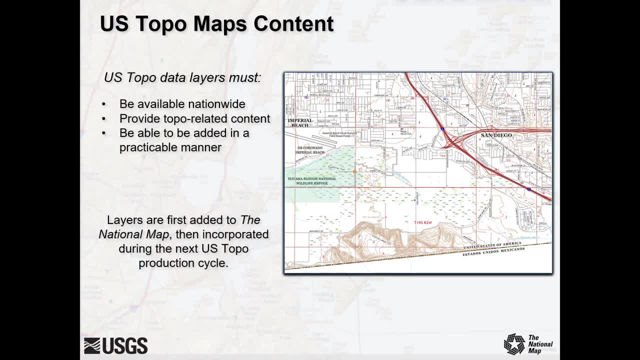 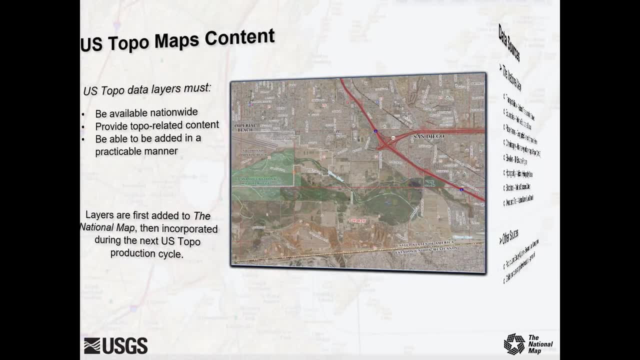 Layers are first added to the national map and are then incorporated during the next production cycle of the US Topo maps. The map layers in US Topo come from a number of sources, as can be seen here. The map layers in US Topo come from a number of sources, as can be seen here. 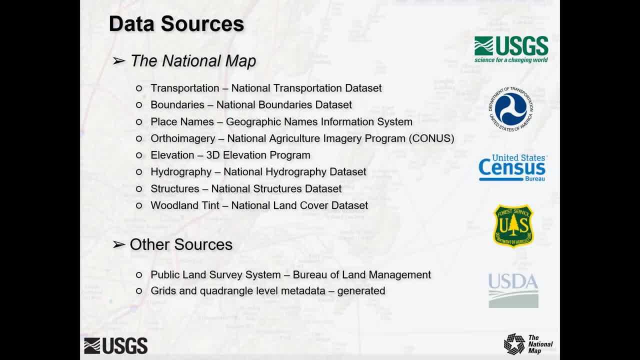 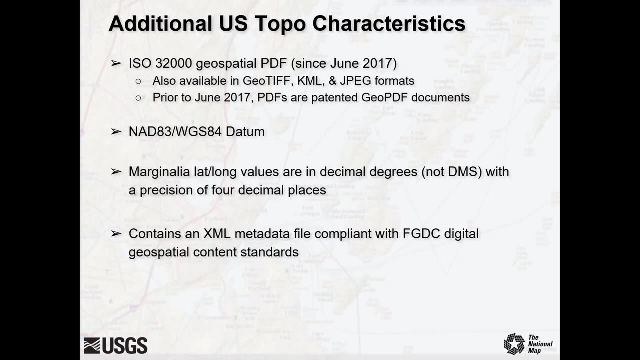 Much of the data originate from within the USGS or through agreements made as part of the national map. For a deep dive into each layer of the national map, please see Lesson 2 of this series. US topo maps can be easily viewed and printed from a normal office computer without specialized software or expertise. 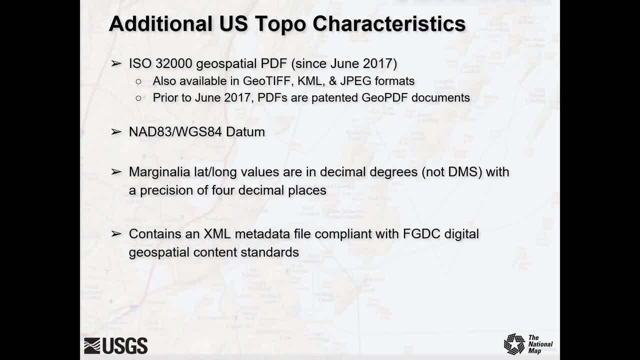 They can be downloaded for free online in a variety of geo-referenced formats. The datum on all US topo maps is North America 1983,, World Geodetic System 1984, and latitude and longitude values are provided in decimal degrees precise to four decimal places. 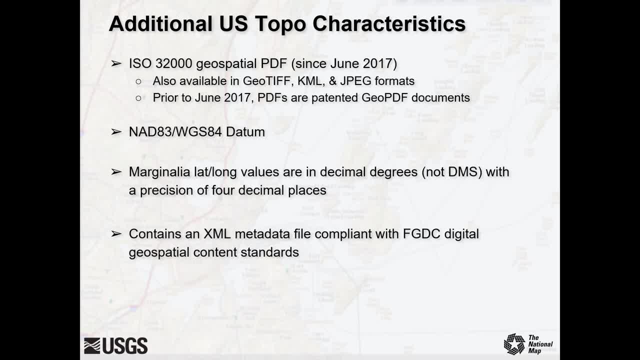 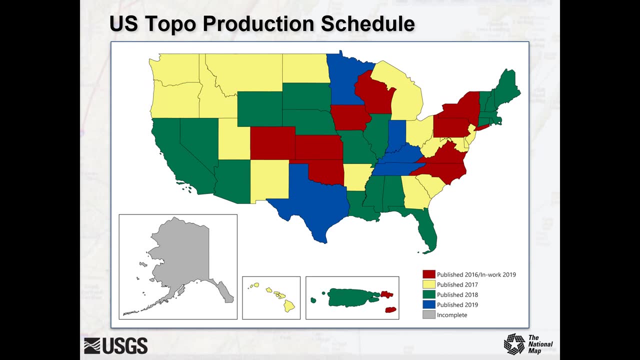 Each US topo map has an attached metadata XML file that describes data sources and production processes complying with federal Geographic Data Committee content standards for digital geospatial data. Starting in 2008,, 2009, and continuing beyond 2019,, US topo maps have been produced on a three-year cycle. 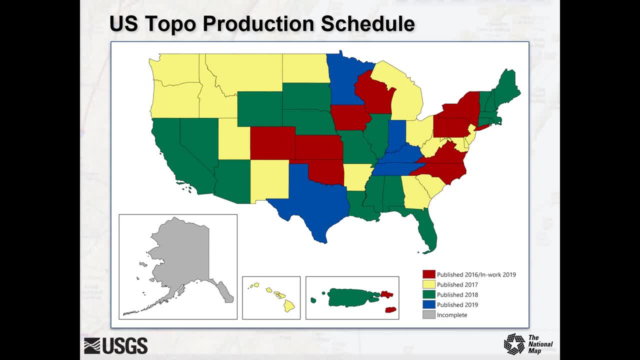 This graphic shows a snapshot of a 2019 cycle where the oldest current US topo maps of the contiguous United States produced in 2016 have been partially replaced by newly created 2019 maps. However, as the map refresh process takes place throughout the entire year, 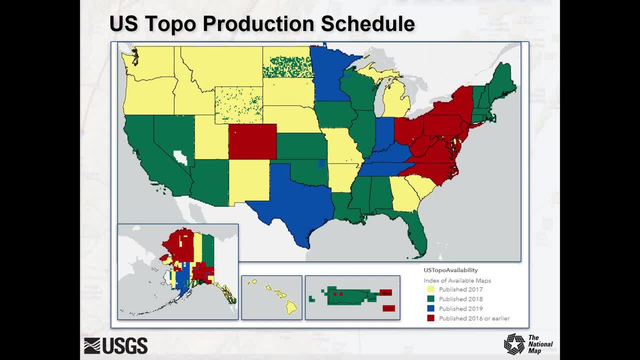 please refer to the US topo availability web service found at viewernationalmapgov if you want to know exactly which regions have been completed at a given time. This is the most reliable source of determining the US topo map date for a particular area of the United States, other than downloading the maps themselves. 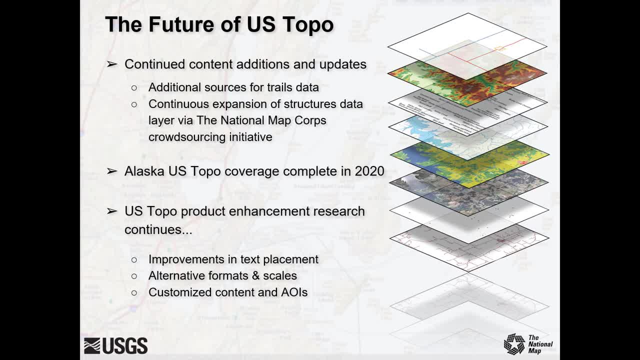 Content, additions and updates to the US topo will persist for the foreseeable future. For example, trails which first appeared in the US topo maps in 2014 will continue to expand as additional data sources become available. Structures will also receive continuous expansions as data is added via the National MapCorp crowdsourcing initiative. 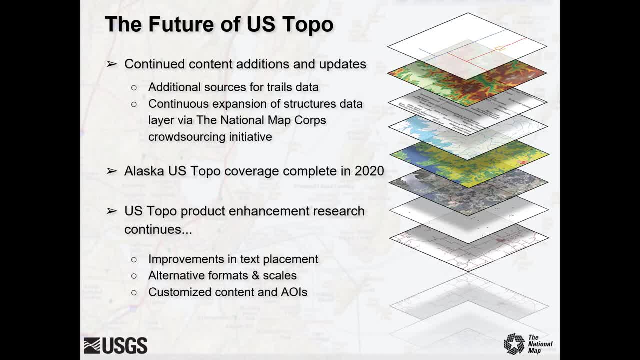 US topo coverage of Alaska will also be completed by the end of 2020.. Finally, research continues into enhancements of US topo products, such as improvements in text placement and providing maps in alternative formats, scales, or with customized content and areas of interest. 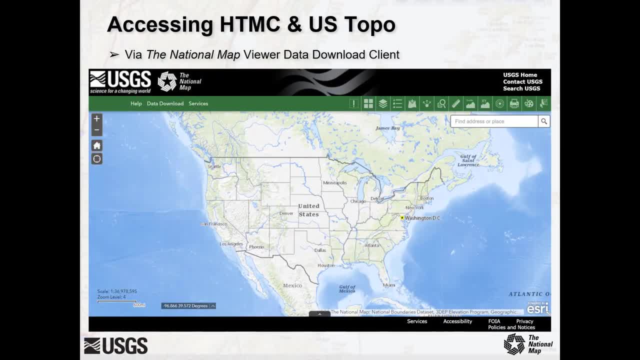 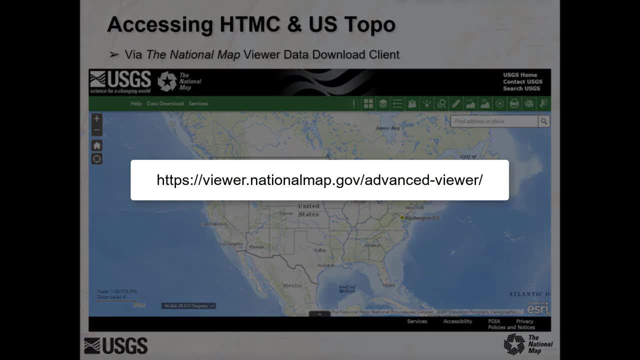 There are multiple ways to access the historical topographic map. There are multiple ways to access the historical topographic map. There are multiple ways to access the historical topographic map collection and US topo products. The first method is to go to the National Map Viewer at ViewerNationalmapgov. forward slash Advanced dash Viewer and click Data Download. 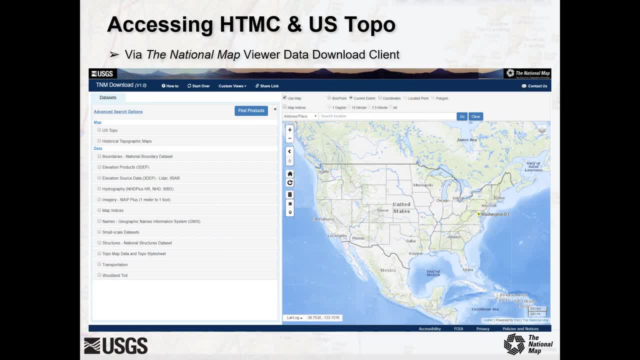 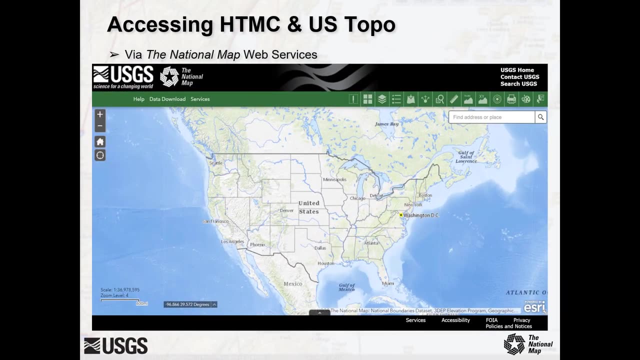 This will take you to the National Map Download data client. Use the map interface to navigate to your area of interest. Check the boxes for US topo or historical topographic maps and click the Find Products button. US Topo data is also viewable in the USGS Topo Basemap. 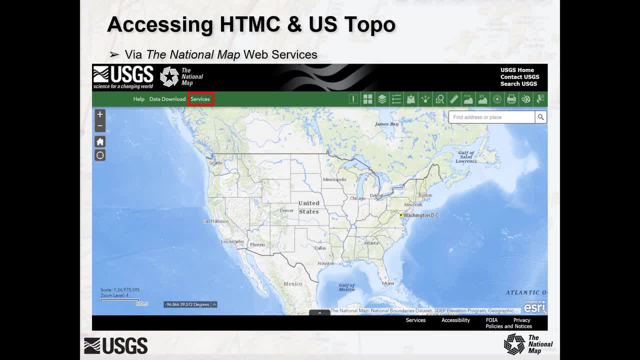 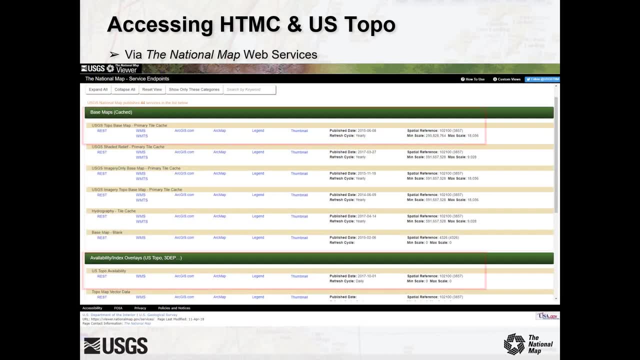 Returning to the National Map Viewer, click Services to view all available services and links. The US Topo Availability Service mentioned earlier can also be found here. Another important thing to note is that most of the vector and raster layers seen on US Topo maps can be downloaded or connected to individually using the National Map Download. 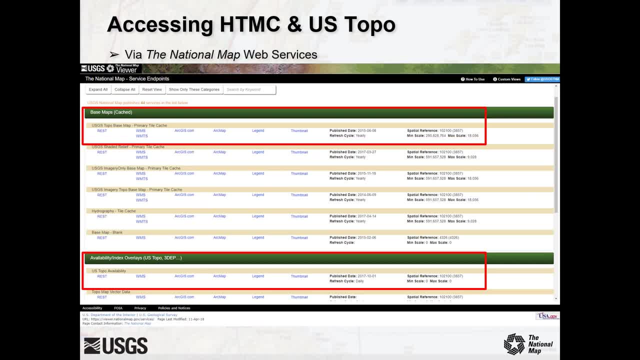 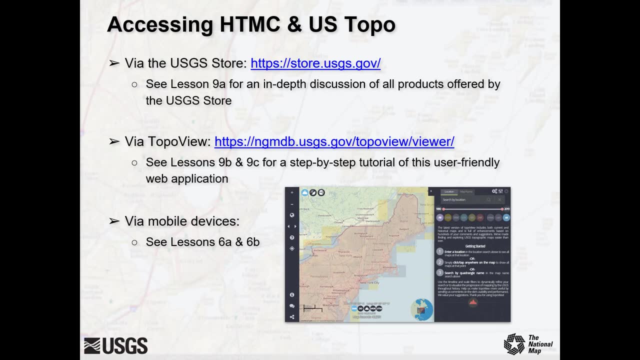 Client, the National Map Services and other online resources. Several of the lessons in this National Map Collection provide details on downloading and connecting to this GIS content. The Historical Topographic Map Collection and US Topo maps can also be accessed through the USGS Store, the Topo View web application and through mobile devices. 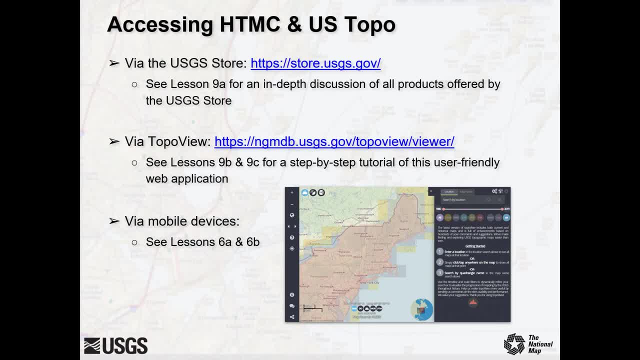 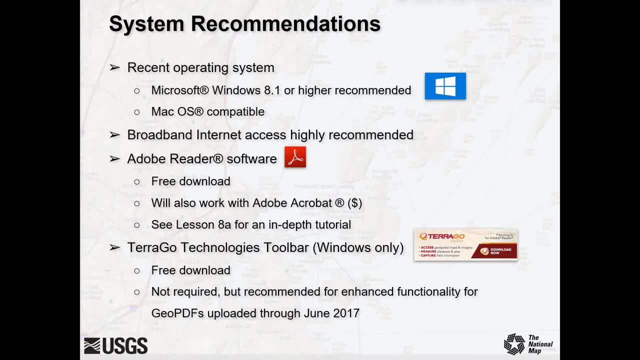 Please see their respective training videos for a more in-depth tutorial. In order to access and view US Topo maps, please click on the top right corner of the screen. For US Topo maps, a recent operating system is recommended, as is broadband internet access. 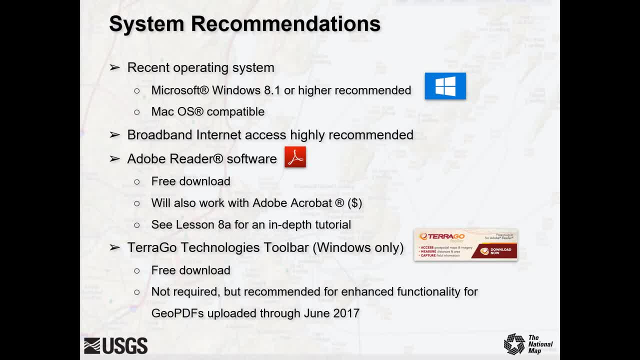 Adobe Reader software or an internet browser extension capable of opening PDFs is needed to view PDF files. Files are also compatible with Adobe Acrobat. Terago Technologies Toolbar is not required, but does provide enhanced functions for GeoPDF maps published before July of 2017.. 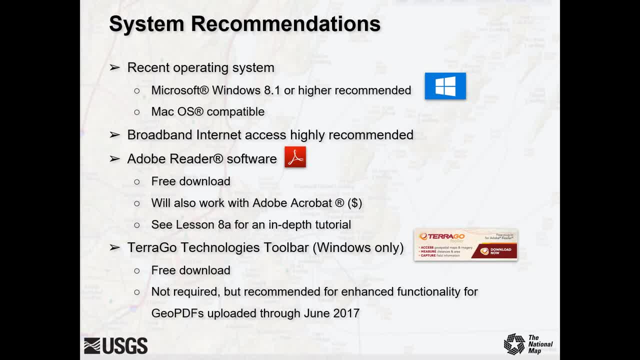 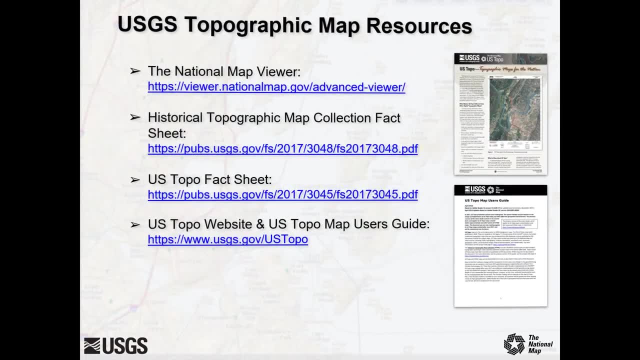 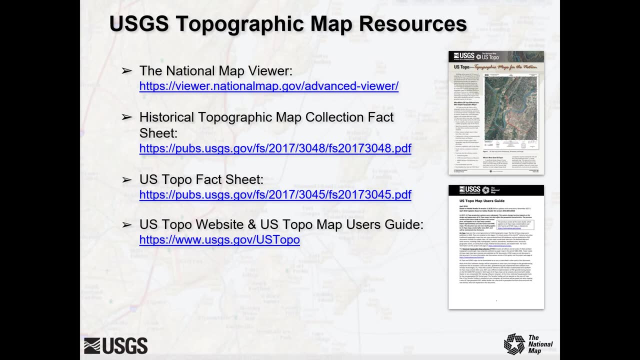 For geospatial PDFs published since that date. Adobe's Measure tool offers similar functionality. Please see Lesson 8a for an in-depth tutorial. For more information, please visit the links provided here to the National Map Viewer, the Historical Topographic Map Collection factsheet, the US Topo factsheet and the